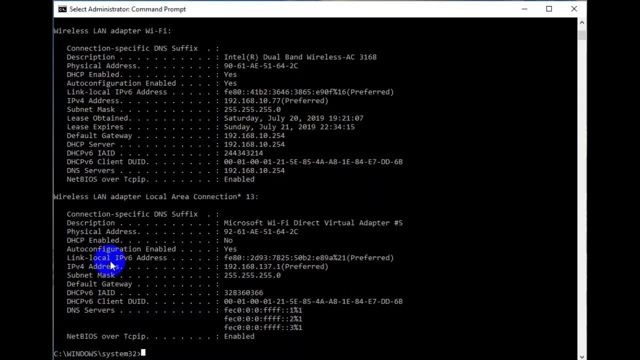 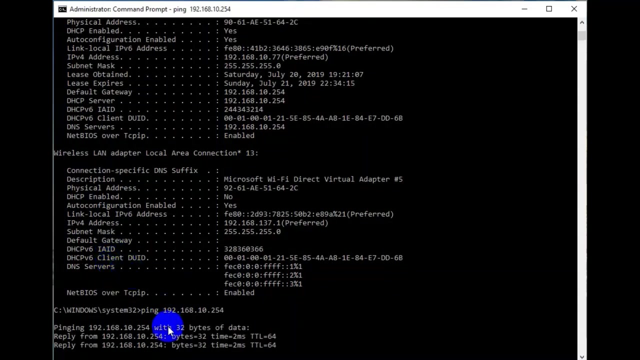 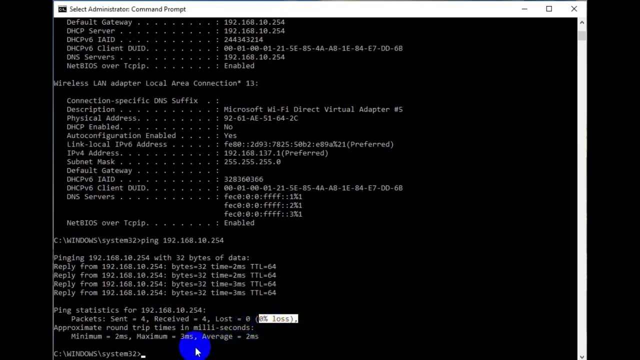 the communication between the device and default gateway. we will ping here with the default gateway. ping our device with default gateway. As you can see, there is a zero percent. It means this is a connection between the device, the with one another on a network. now let us move to tracer command. 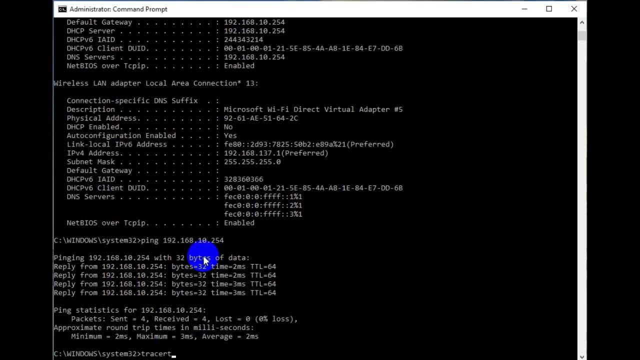 basically, tracer command is used to show several details about the path that a packet takes from computer or device. you are on to whatever destination you specify. in simple words, tracer command is used to show the several paths or the routes from a computer to a device to whatever destination you specify. 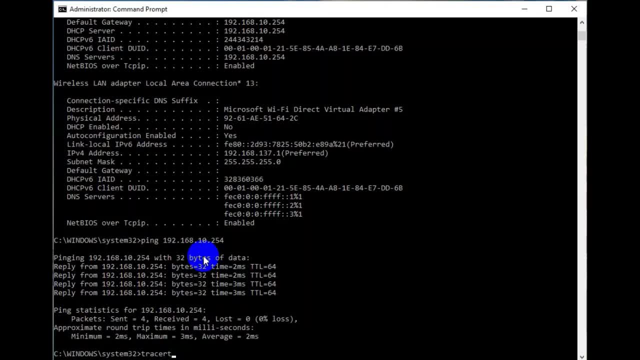 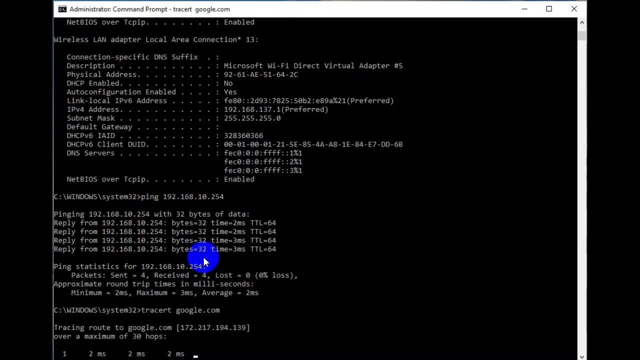 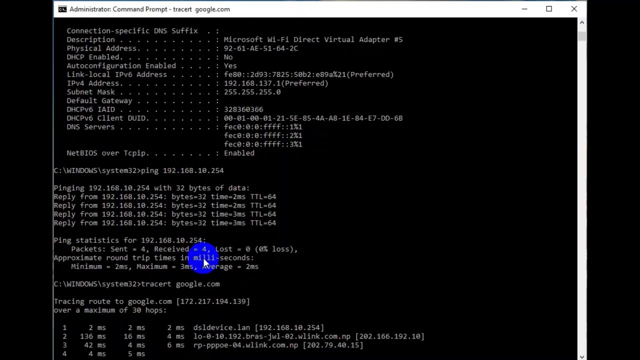 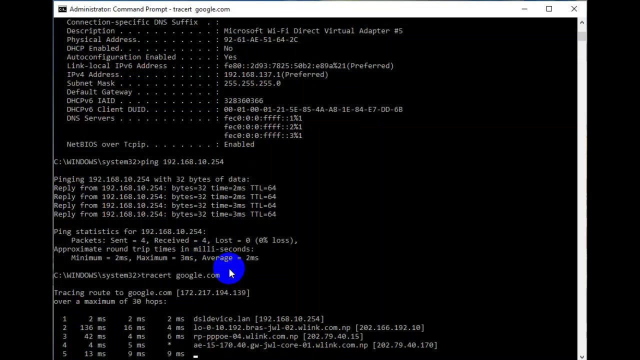 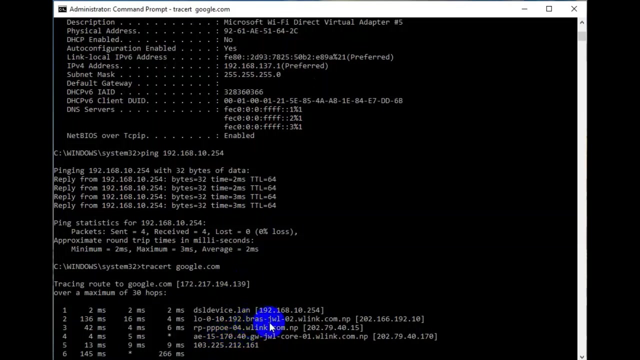 let us take an example. here I am tracing googlecom for young tracer space. here you can see the several details about the path and we may see that at each location. by this tracer command we can subscribe each other�� to the page and tinker icon. 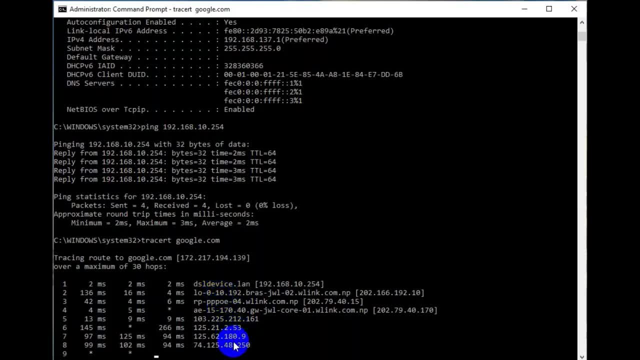 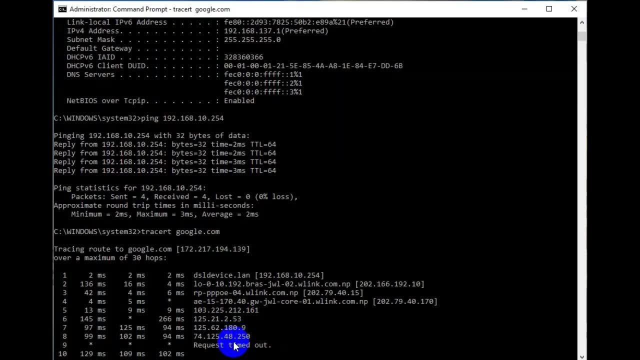 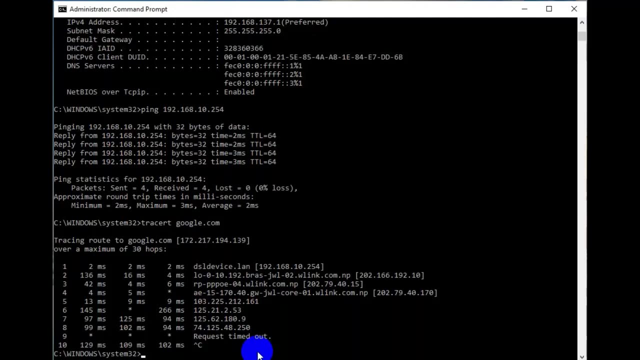 all of the access details are on your screen. you can use a password, type the topic you keep in, though yournt use to select partido. battles list can see the several paths, several details about the path that a packet takes from computer or device. Now let us move to NSLOOKUP command.